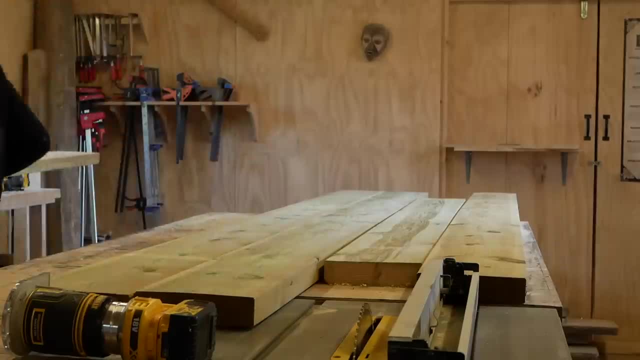 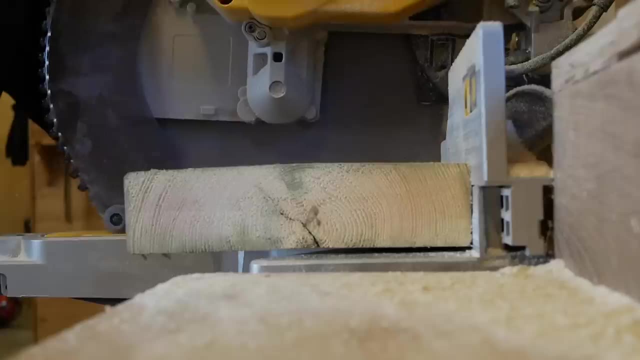 it a secret. It almost seemed like he felt bad at how easy it was. Now, my grandpa could easily make a whole set of outdoor table and benches in a day, and he did not do any sort of marketing. It was all through word of mouth, So he definitely knew what he was talking about. but 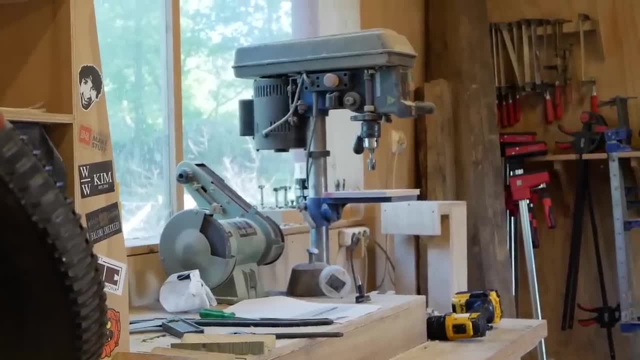 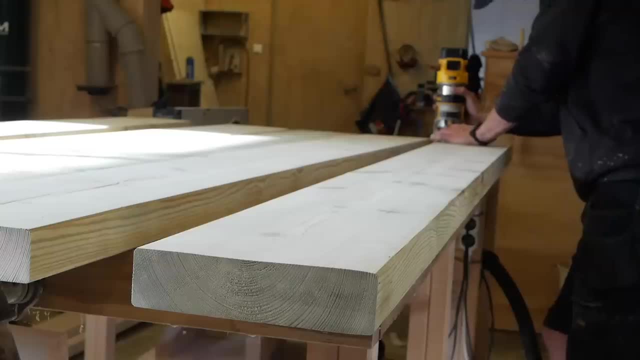 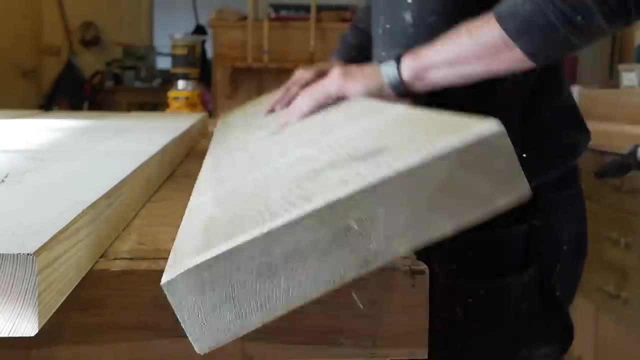 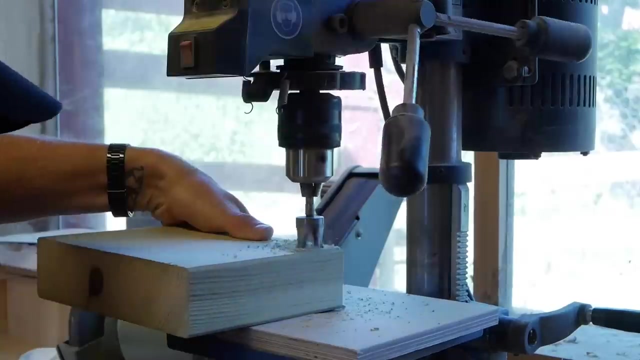 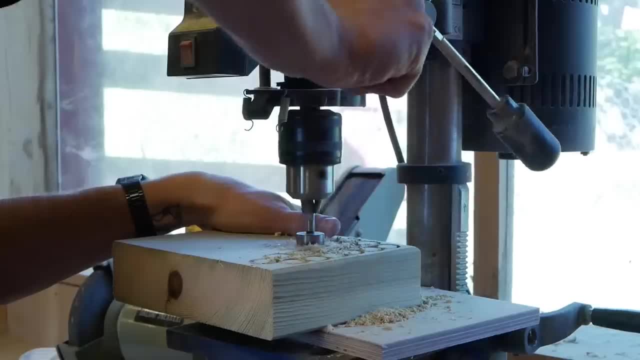 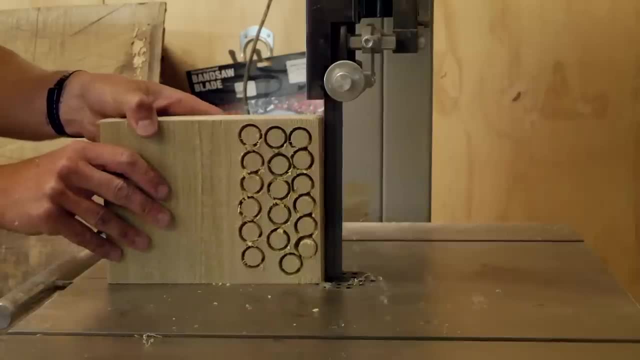 I was not interested in making money on outdoor furniture. I was not interested in making money on woodworking. I pictured myself as a Sam Maloof kind of guy making high-end furniture or making lots of money per sale instead of mass producing. I did not want to make the same things twice. 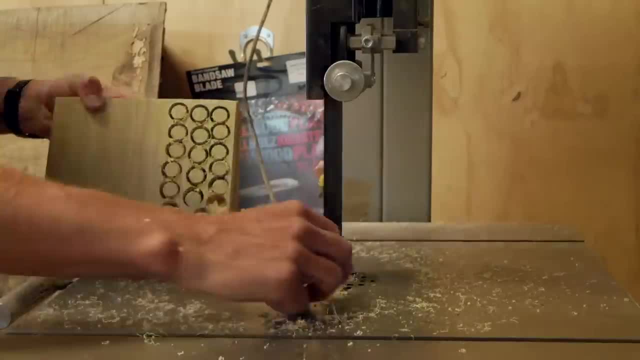 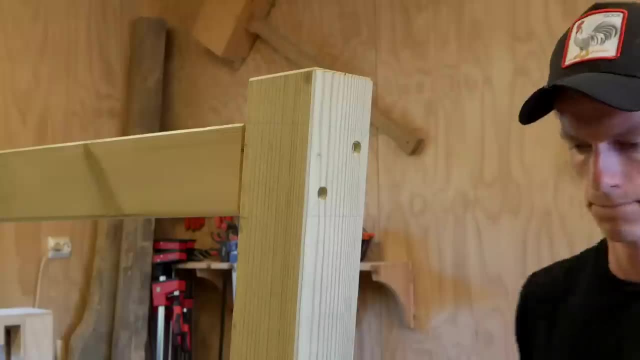 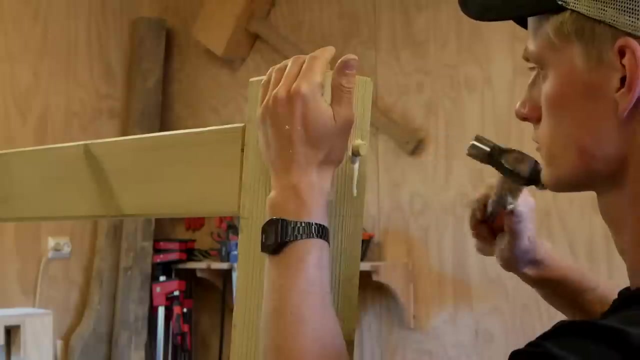 and I was picky about the projects that I took on. Now I think that it's definitely possible to make money that way, or I know that it's possible. So if that is your dream, absolutely go for it. That's where I want to end up as well, but that is not where I'm at. 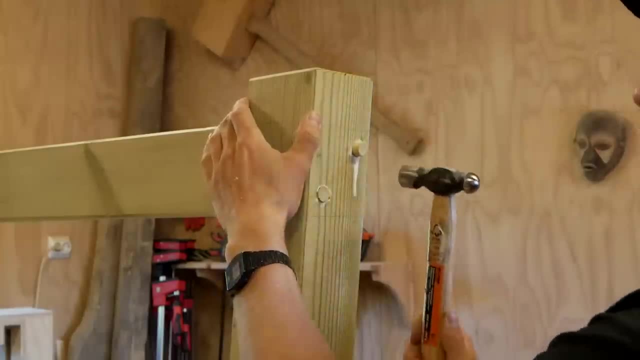 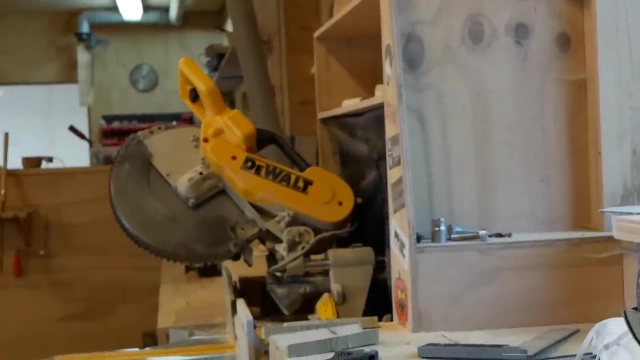 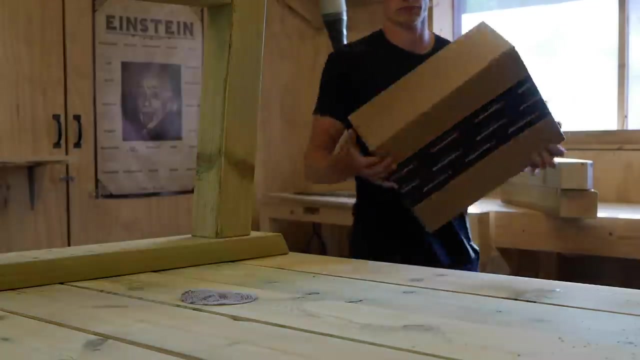 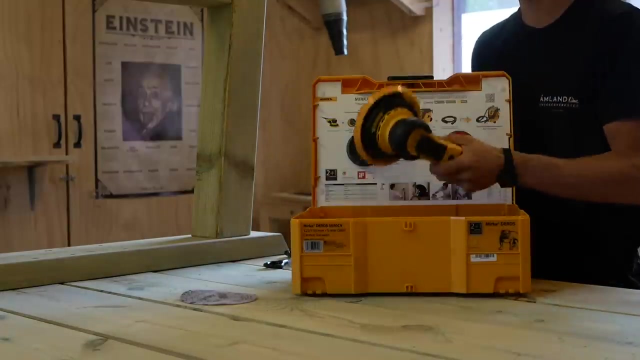 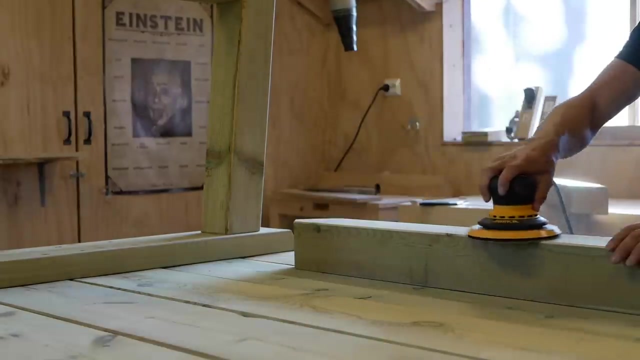 yet, and it hasn't worked for me up until this point, and I'm soon going to tell you why. So, instead of listening to my grandfather, I made some pretty decent furniture that I spent a lot of time on and I sold way too. 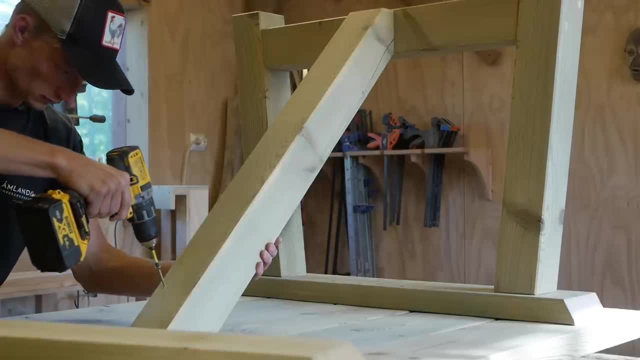 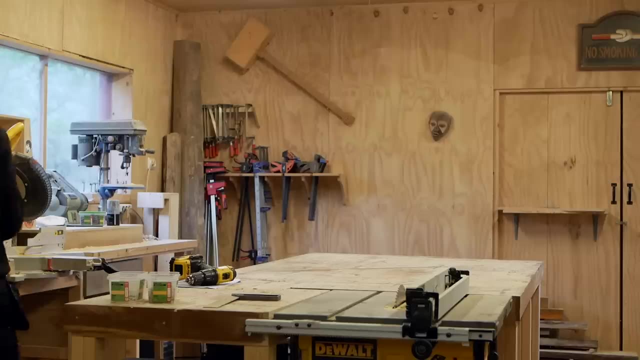 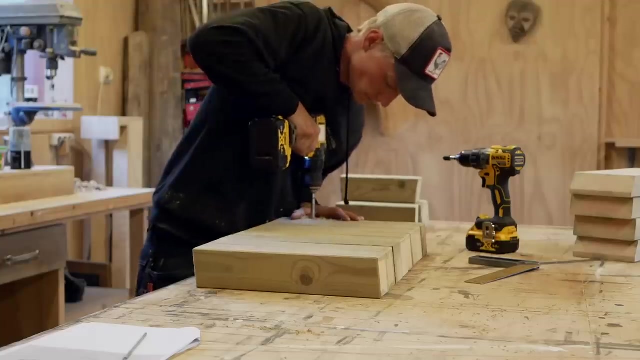 cheap because I did not feel good enough to charge high ticket prices. So what ended up happening was that I spent a lot of time trying to make the perfect furniture, but made little money. My hourly rate was terrible. For example, I spent five weeks of full-time working on a project. 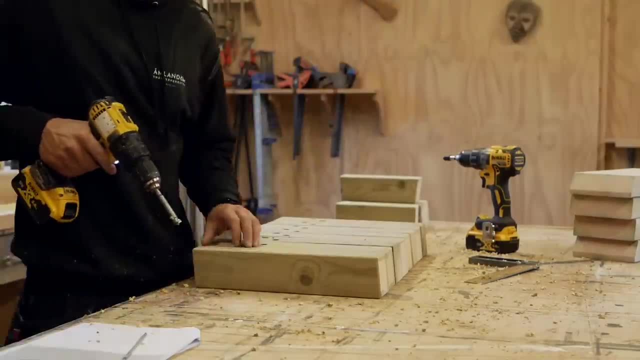 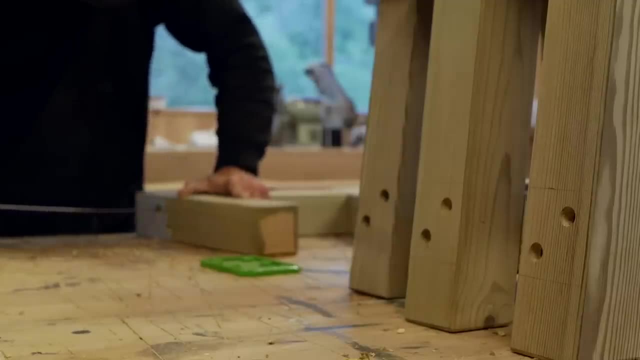 then I made $1,500 profit from, And, of course, this frustrated me a lot. I had the dream of making a living as a furniture maker, only building projects that I was passionate about, but I did not manage to get into that. 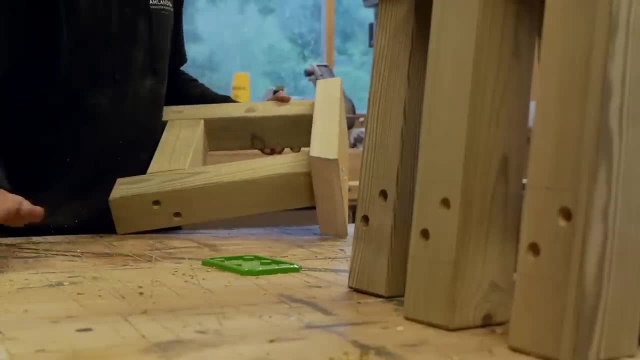 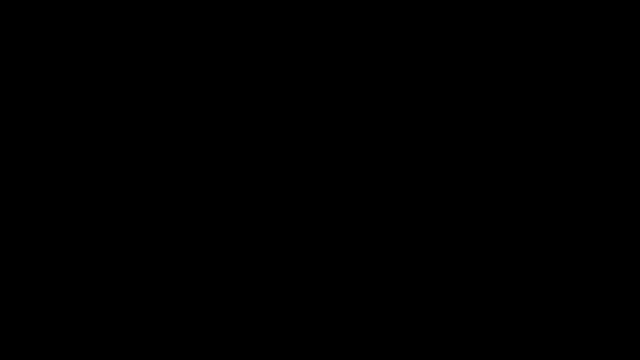 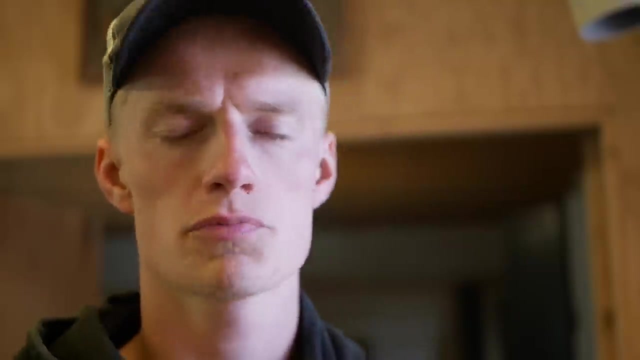 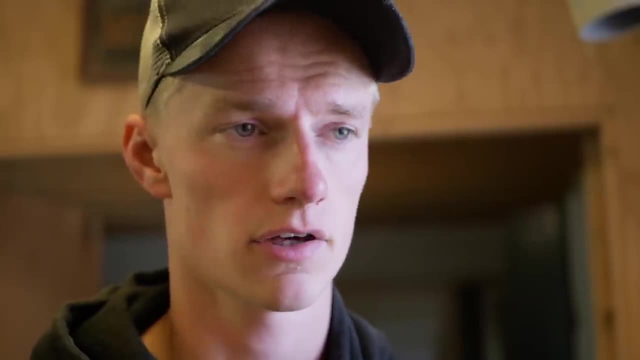 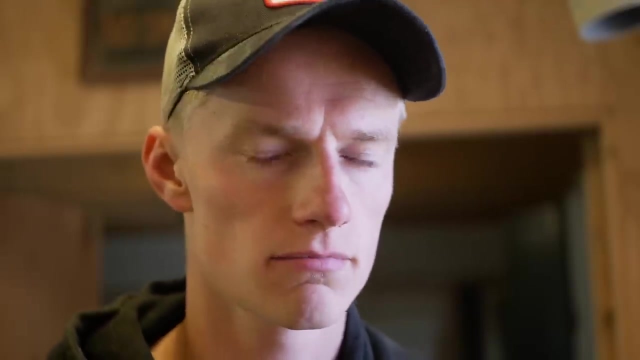 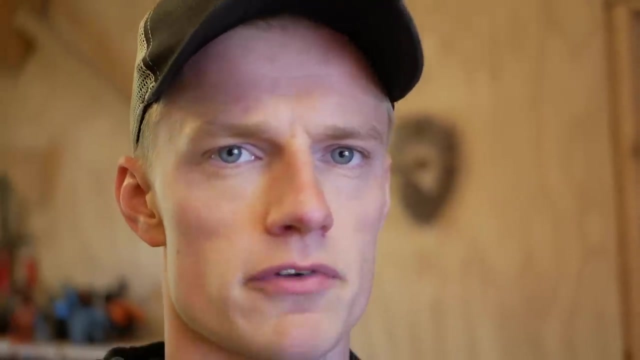 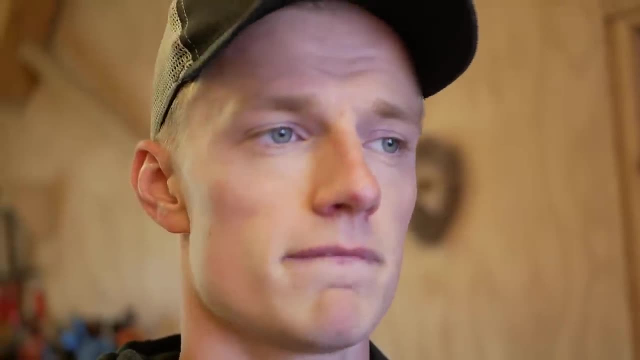 to have to make a lot of money from it. So you're going to have to make a lot of money from it. So to charge a lot of money for it, the precision and everything. it has to be just dead perfect. 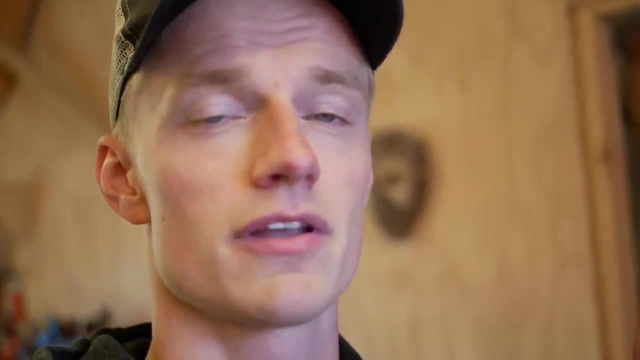 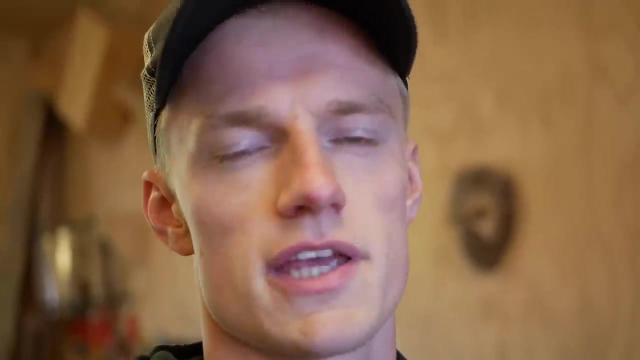 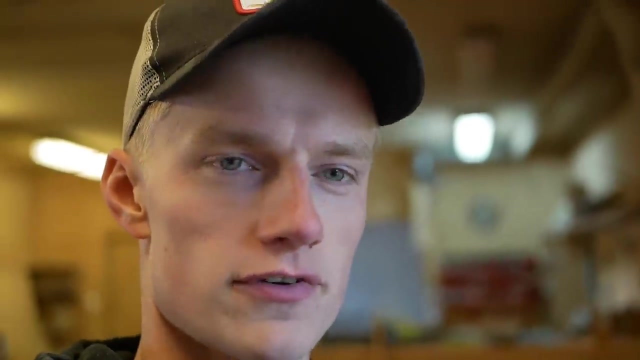 It has to be at a high level, So you need to have a high skill level, but also your tools and machines will have to be very, very precise, And that just wasn't the case for me. And then, finally, I tried to sell things that I want to make instead of making things that people want to buy. 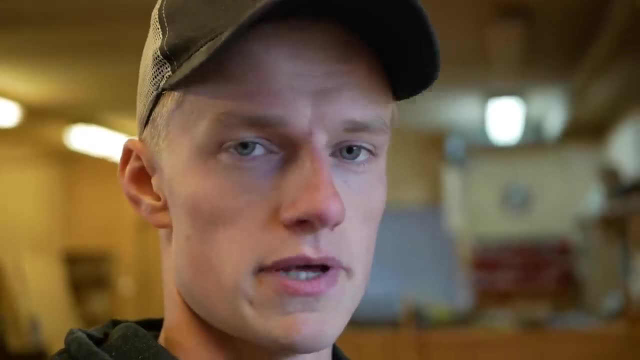 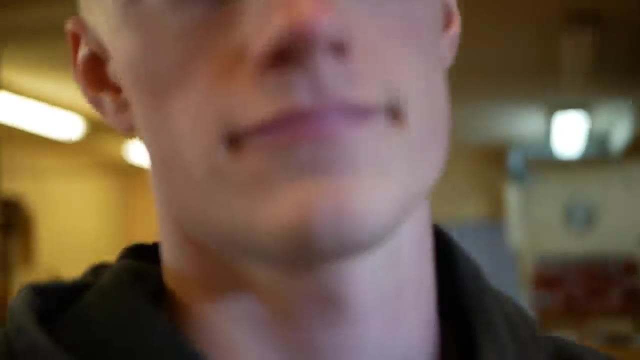 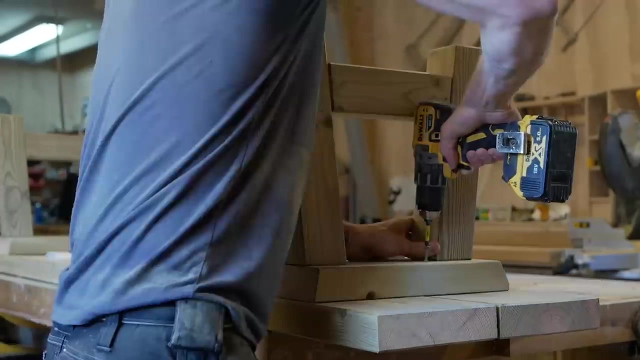 That's not a good idea. You want to find products that people are willing to pay for, and then you have to make that and sell that. So after I realized this, I sat down and started designing an outdoor furniture set. The main points that I focused on were that it had to be. 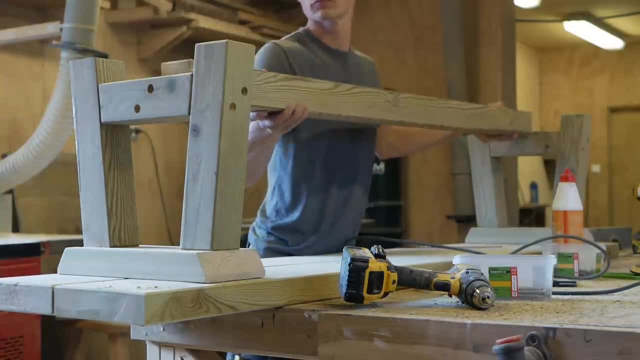 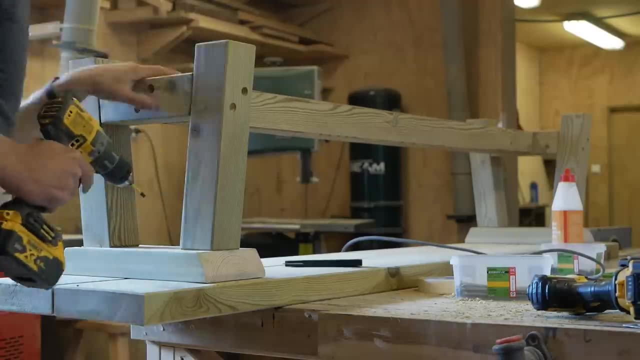 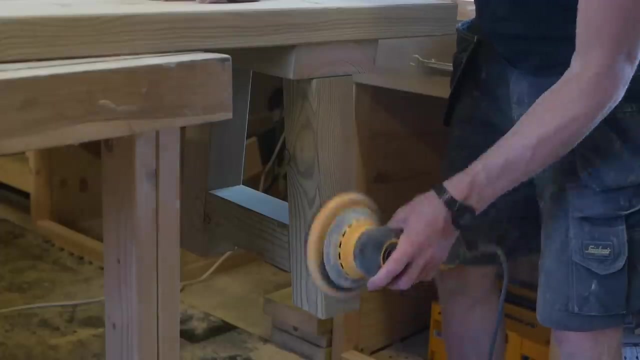 durable, solid and easy to build. So no complicated cuts, just simple techniques and joinery That was easy to replicate. At the same time, I wanted it to look good. I wanted to have a clean, modern design, So that was the balance that I tried to find. 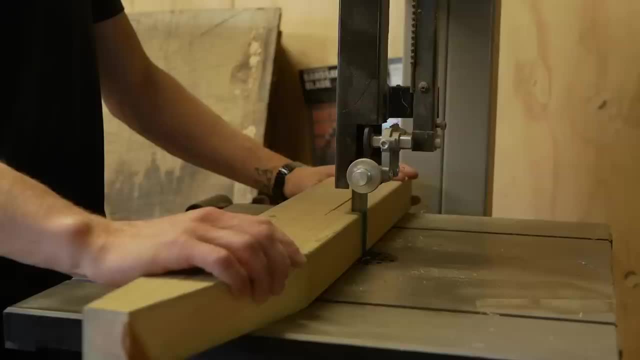 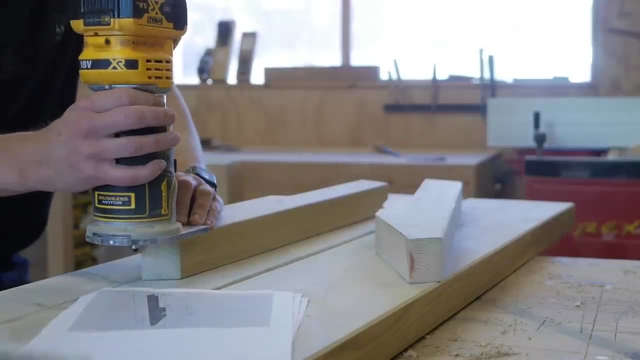 You can't express everything in a very short space. You have to be consistent and just feel comfortable about it. It was very easy. I didn't even have to be tired after the first six months, so I was able to sort it all out. 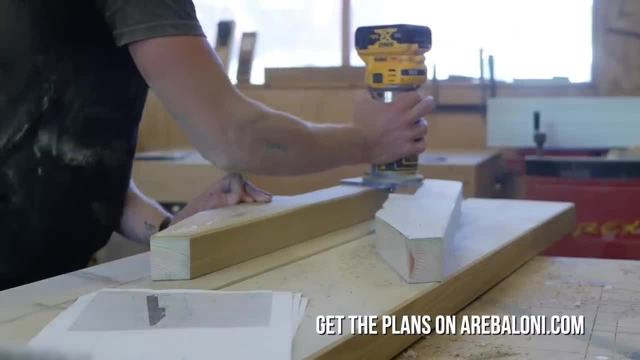 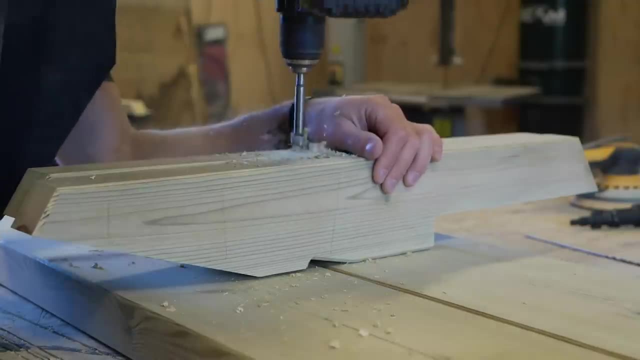 I did the same thing for the first year and I did the rest of the rest of the year. I had a lot of people come in from all over the world and someone said that if I wanted to sell furniture then I could sell the furniture to them and sell it to a big company. 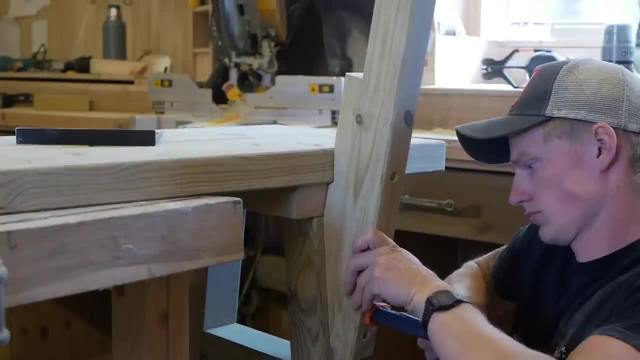 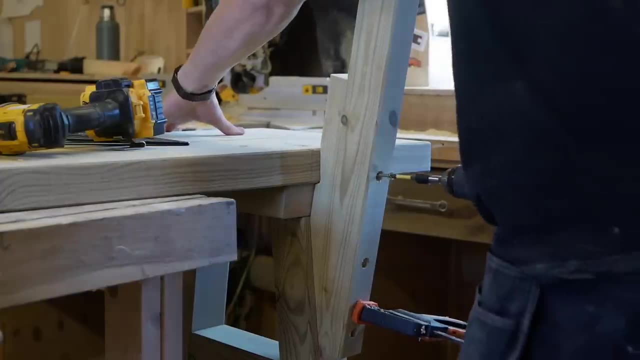 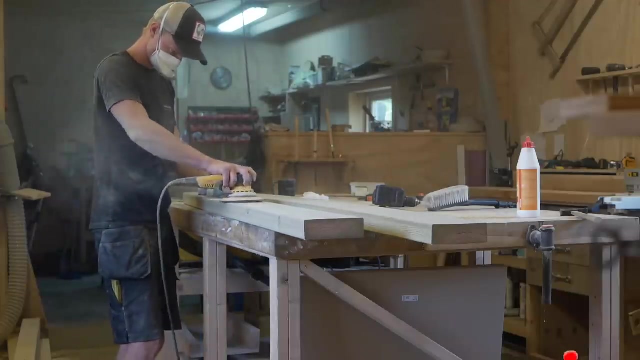 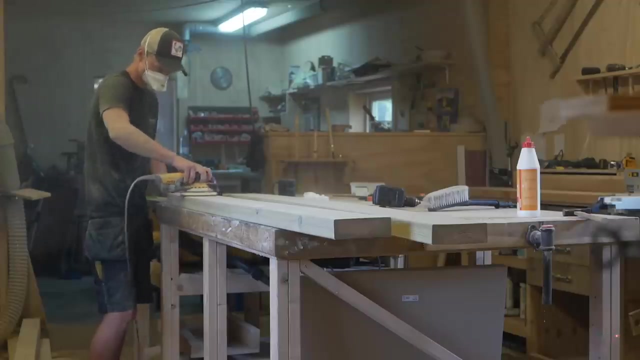 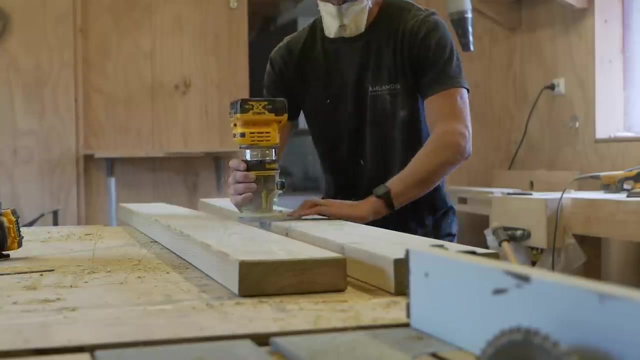 So that worked out. I didn't feel like it was in a limited mass scale. I didn't feel like it was in a limited mass scale. I didn't feel like it was in a limited mass scale. Thank you. 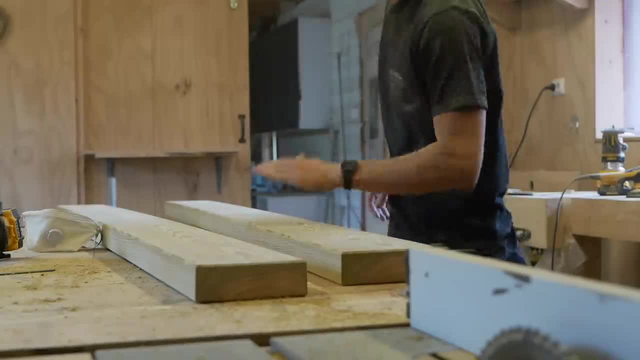 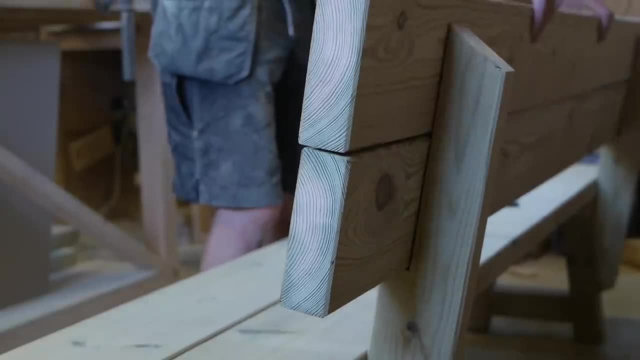 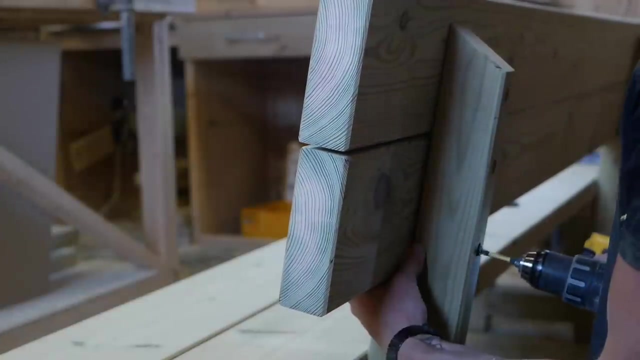 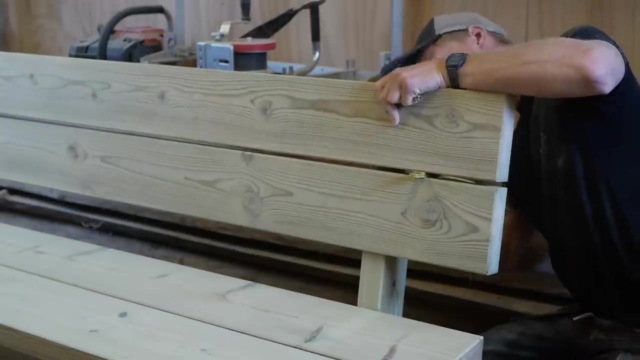 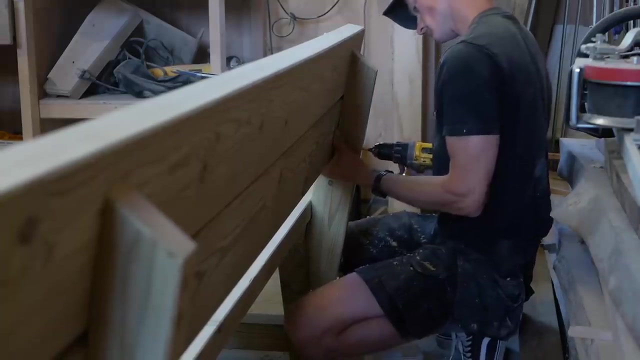 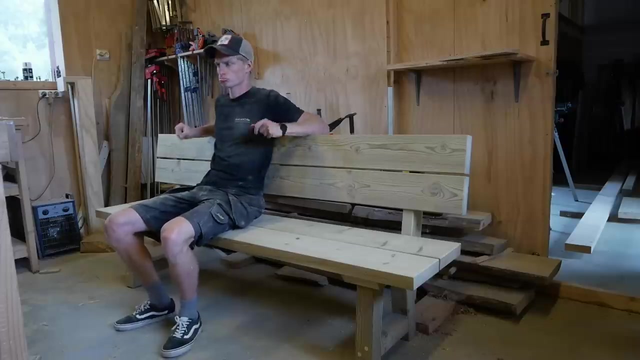 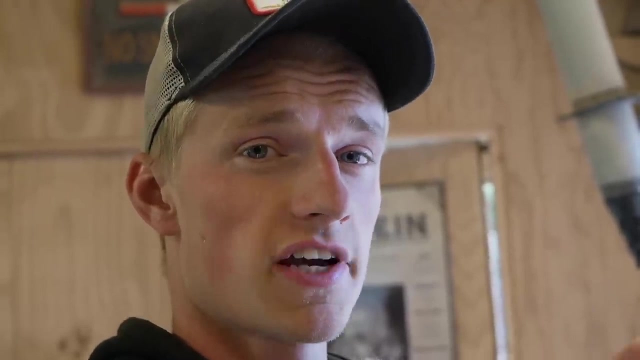 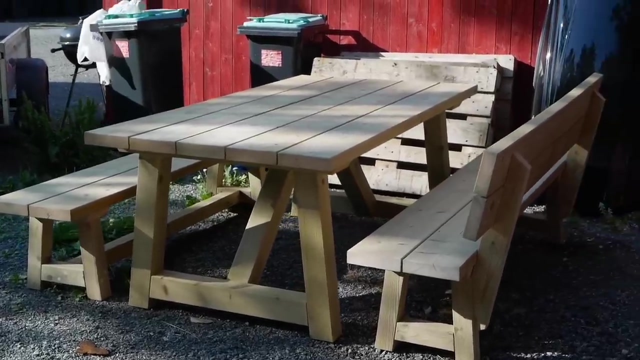 Thank you. Okay, guys, so I just finished up the outdoor furniture set just a couple of minutes ago. Let's go outside and have a look. As you can see, this is pressure treated wood and I have not finished it, And I'm actually not going to either. 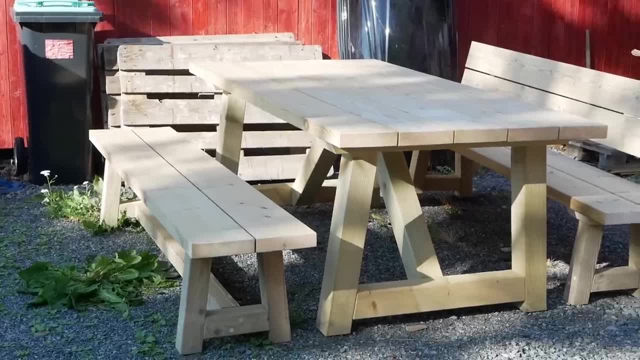 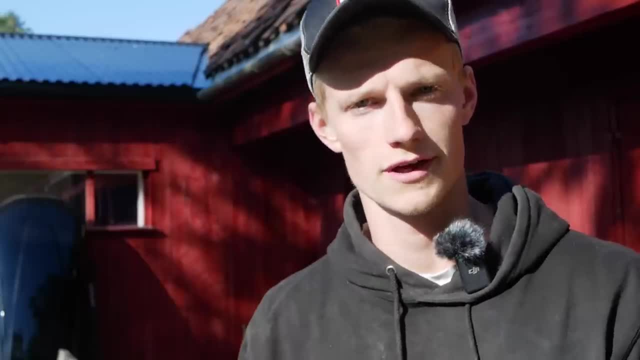 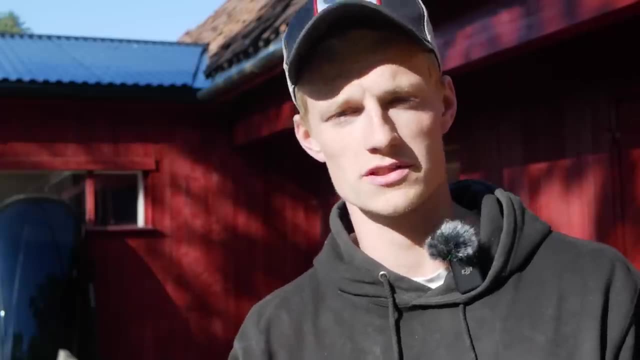 I'm just going to sell it as it is, And this was actually part of my grandmothers Grandfather's philosophy. He told me that if people want to have the outdoor furniture a different color, they are most of the time happy doing it themselves, instead of paying me more money for me to do it. 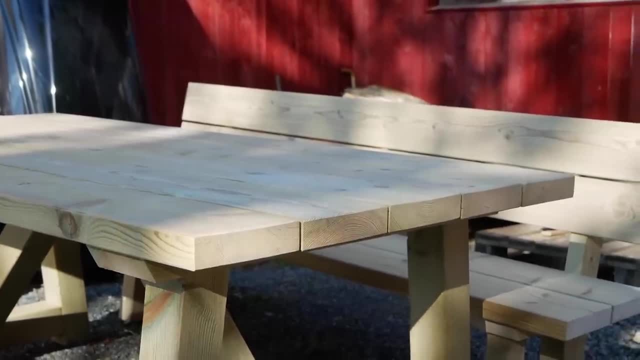 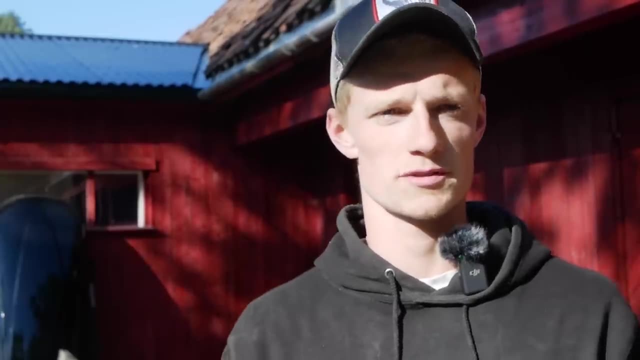 And he said: if you are going to finish furniture, you're going to spend half the time finishing the furniture instead of actually building the furniture. And this does make sense to me, because I spent a lot of time finishing that outdoor dining table that I made in the previous video. 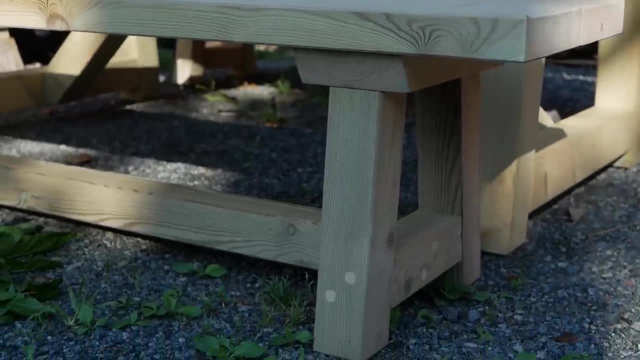 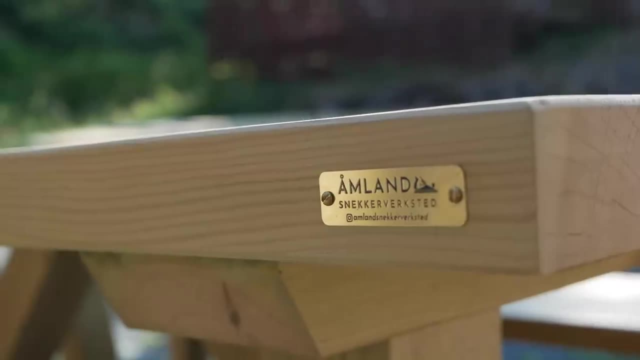 And this outdoor furniture set can just be as it is. It's pressure treated wood, It looks pretty good And it's durable as it is. So now you're probably wondering: do I have any proof that I will make money from this? 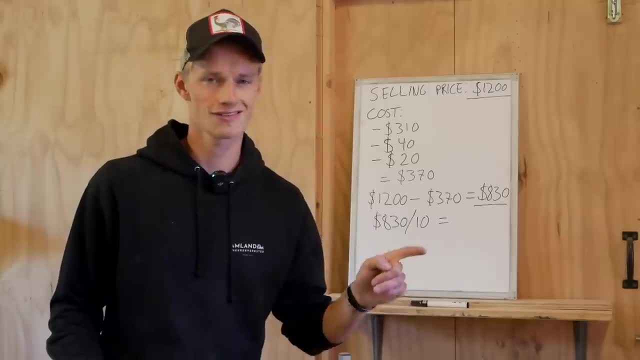 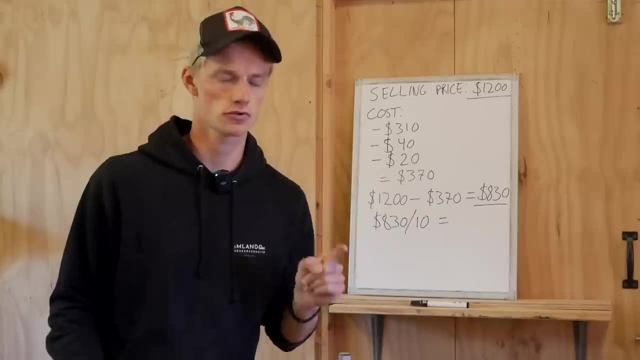 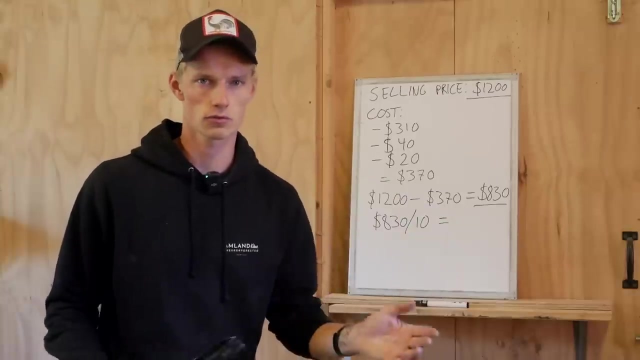 Well, yeah, kind of Already before publishing this set I have sold for $3,600.. I'm selling them at $1,200 per set. As it is Two meters long. Of course the customers can have it longer or shorter if they want to have it customized. 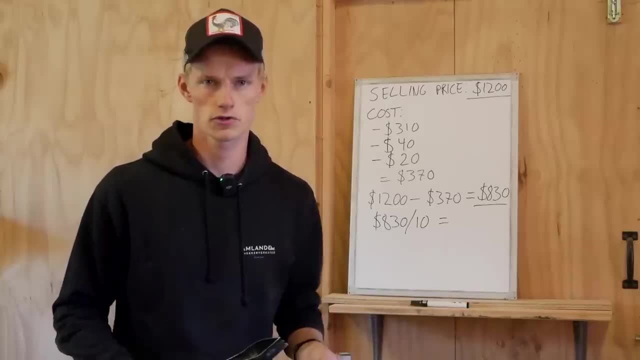 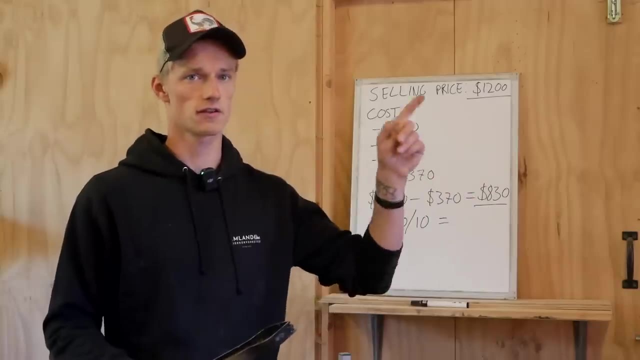 That's part of the reason why people will want to buy from a furniture maker instead of just at a shop. They can get it the size they want, of course, But at two meters I'm selling them for $1,200.. So now let us have a look at the hourly rate. 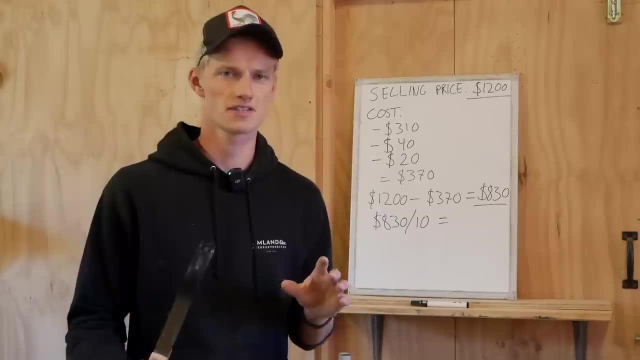 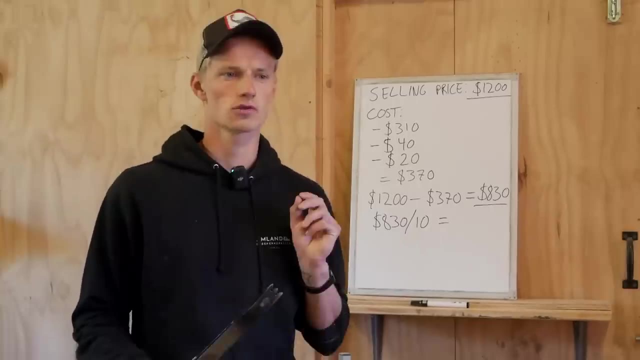 The first time I made this outdoor furniture set, I spent 12 hours making it, And that is with making all the templates and a bit of extra work Having to figure out everything, So I'm confident that I can do it in 10 hours. 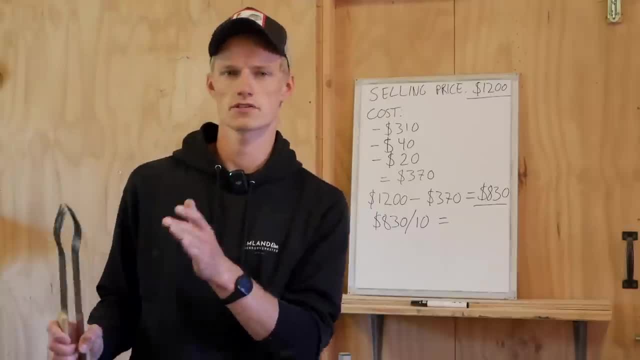 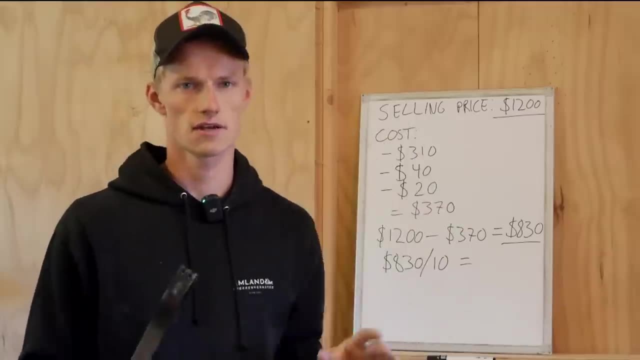 I feel like I can do that pretty easily. Of course, it's all just basic cuts and screws, So it doesn't take very long. So that is both the benches and the table in 10 hours. So the selling price is $1,200. 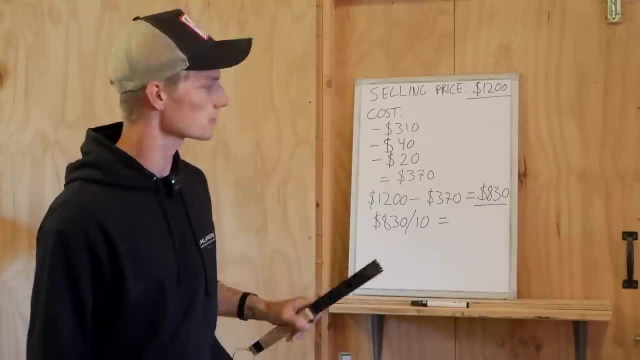 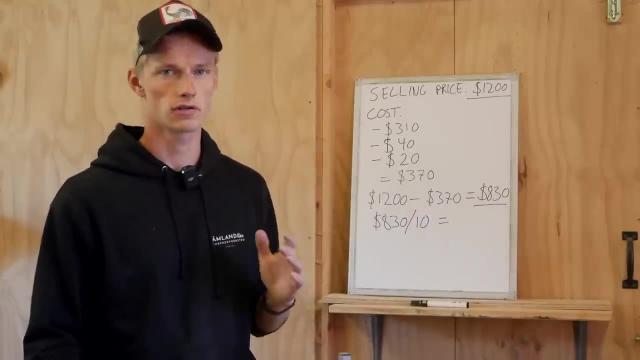 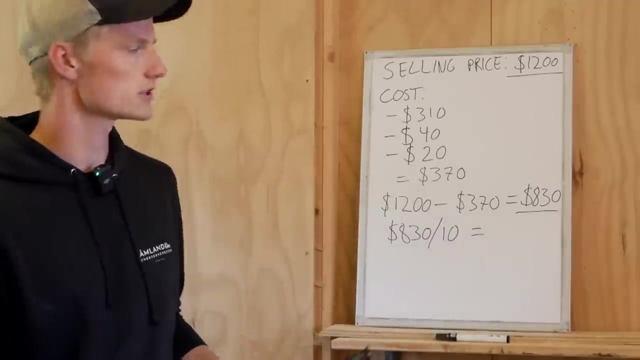 Material cost was $310. Plus around $40 for screws and $20 for samplers, Sandpaper and glue, things like that. We're just going to add about $20. So that is $370 in cost. So $1,200 minus $370 is $830 in profit. 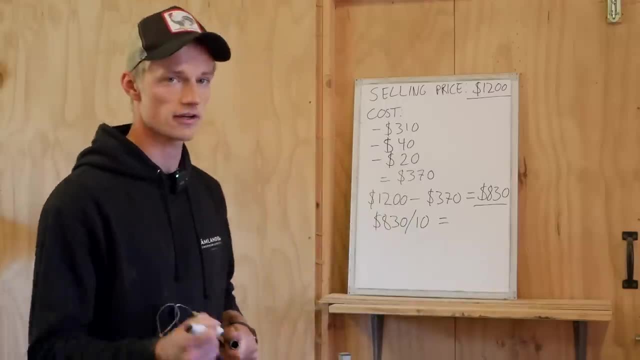 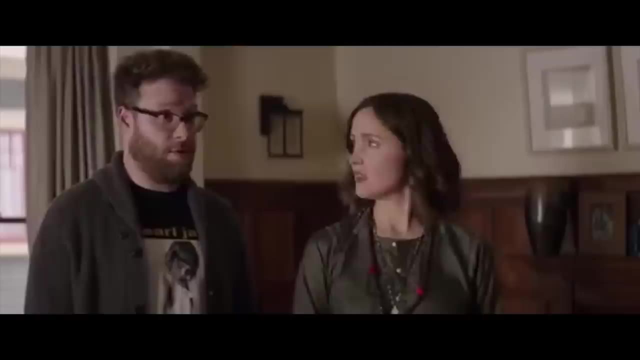 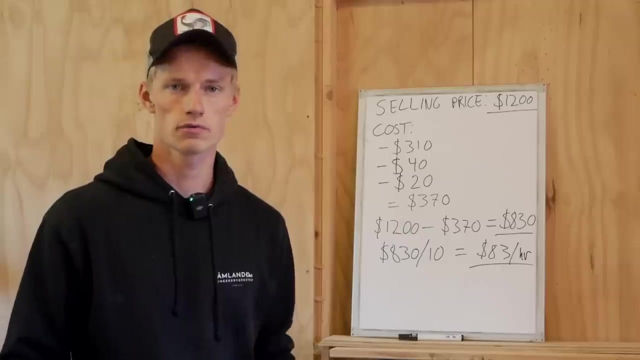 And of course, $830 divided by 10 hours is $83 per hour. You're incredible at math, So of course that is going to vary if that is a good salary or not. For me, where I'm from and my age, that is very, very good. 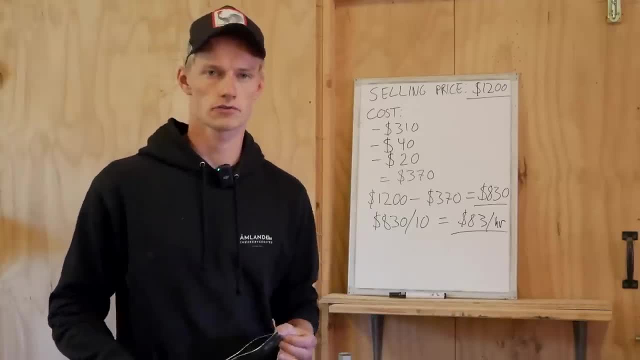 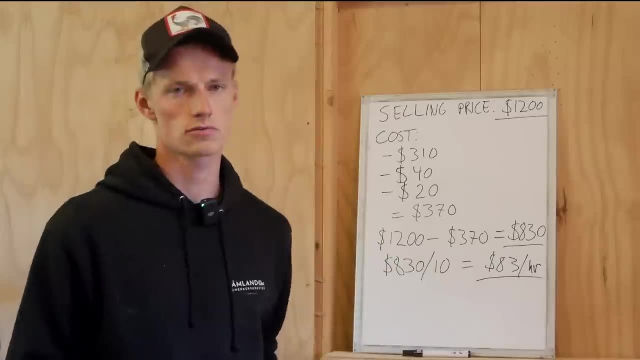 That is way more than I'm making in my day job as a construction worker. So in just 10 hours- that is one long day, or at least in a weekend- I can make $830.. Now for the marketing part. I will use my Instagram. 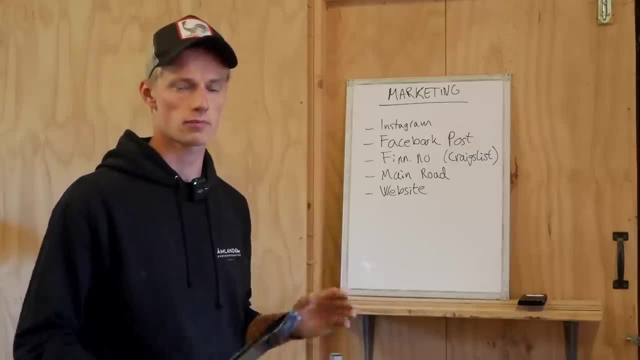 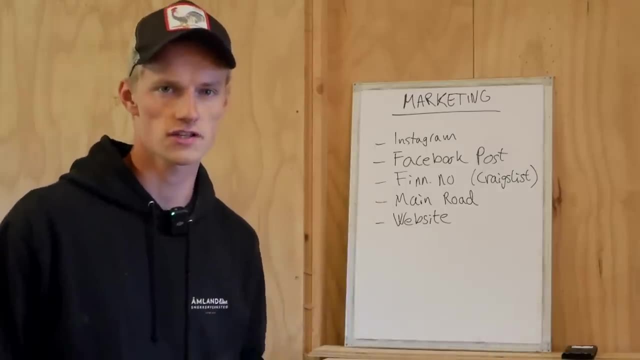 I'll also make a Facebook post on my private account that I'll post and share, And then I will also put it up on finno, which is a Norwegian version Of Craigslist or Etsy, And then I'll also put a set out by the main road that people can see when they drive by. 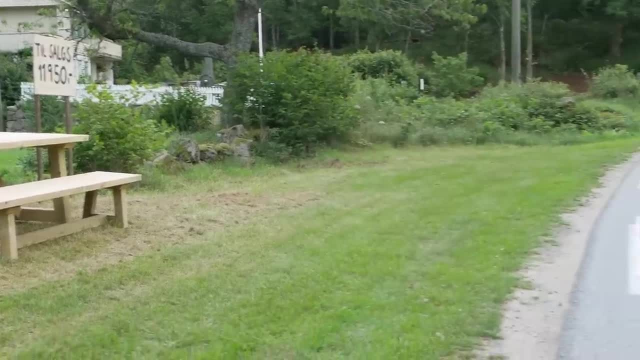 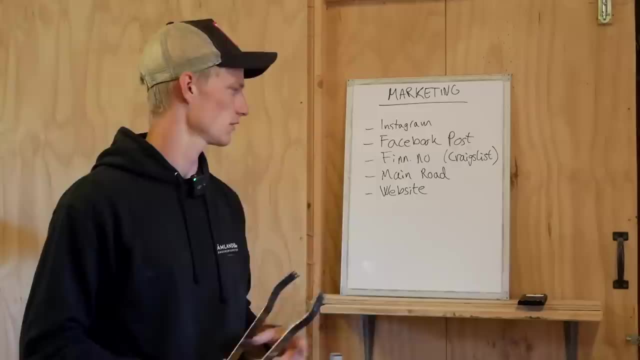 With a big sign that says for sale, And I'll also have a small post poster with some information- contact information, price, things like that. Then I will have a website where it will be easy for people to go and pay an order.